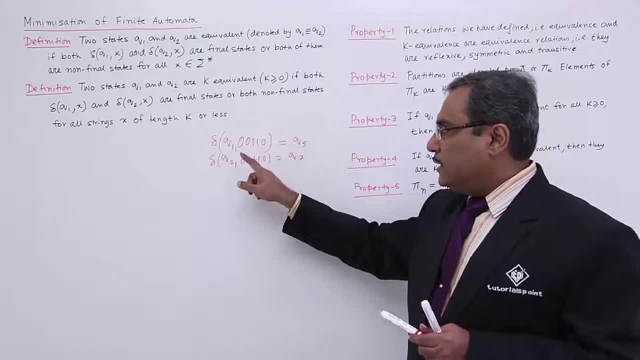 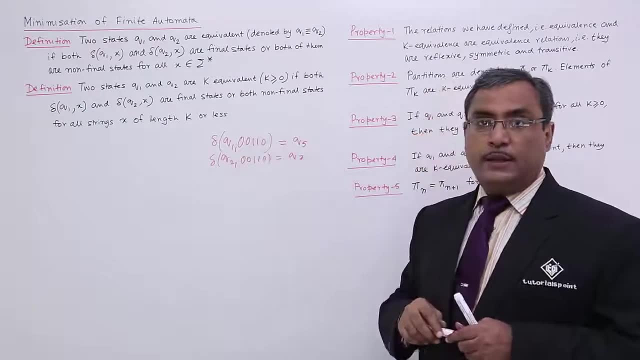 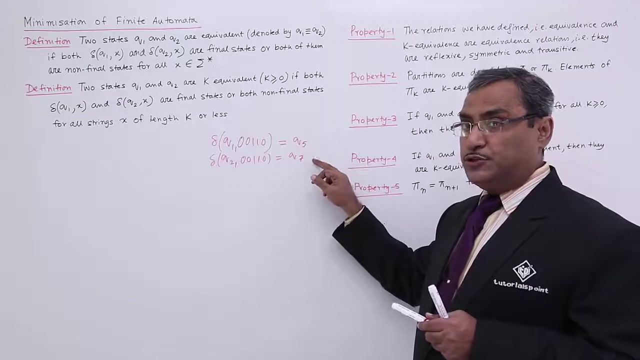 are the final states, then I shall say this: q 1 and q 2 are equivalent, if it is possible, for all possible input strings. Otherwise, if I find that q 5 is a non-final state and q 7 is a non-final state, if it is so, and if it happens, for all possible input strings. 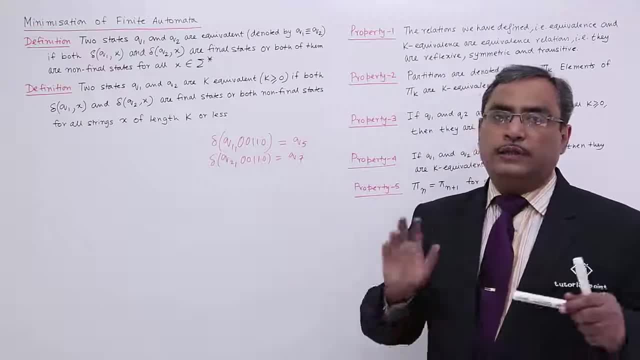 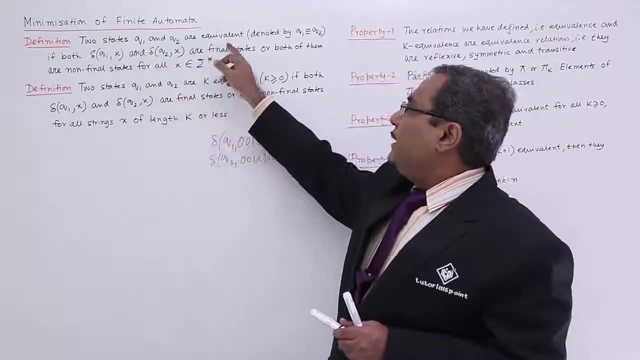 then we can say that q 1 and q 2 are the equivalent states. So it has been depicted here. Let me read that one again. Two states, q 1 and q 2, are equivalent, denoted by q 1 equivalent q 2.. If both delta q 1- x. 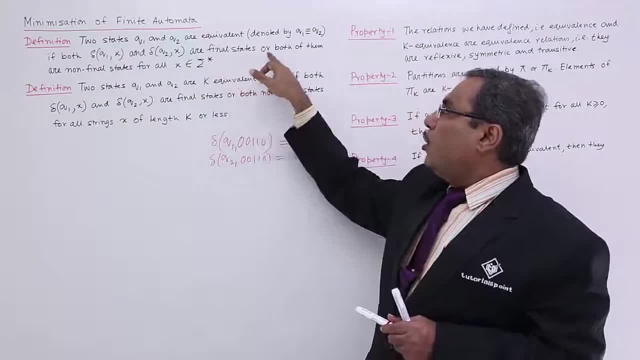 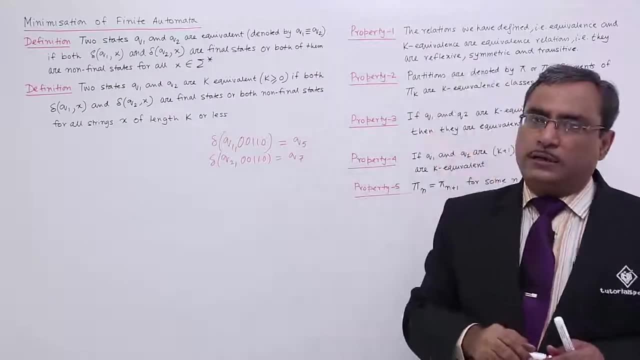 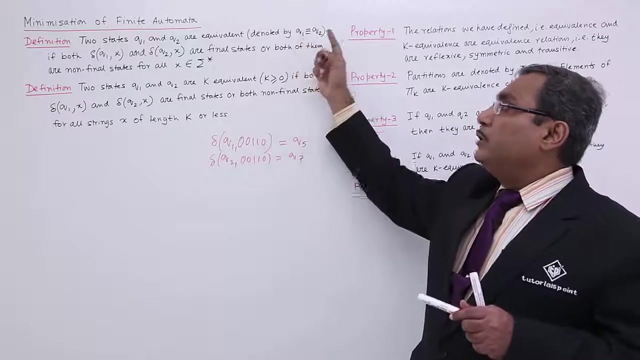 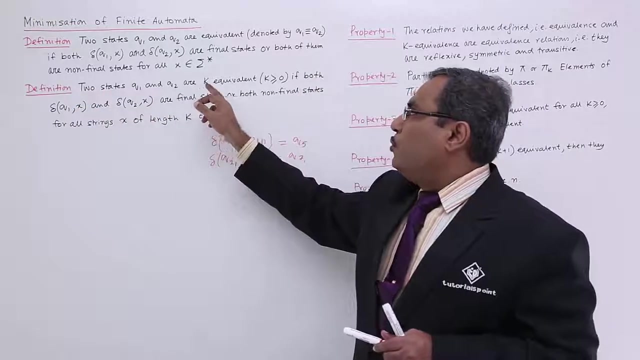 and delta, q 2, x are final states or both of them are non-final states. for all x belongs to sigma star. So that is the proof to have between q 1 and q 2 whether they are equivalent or not. So if we have two states, q 1 and q 2, are k equivalent where k is greater than equal. 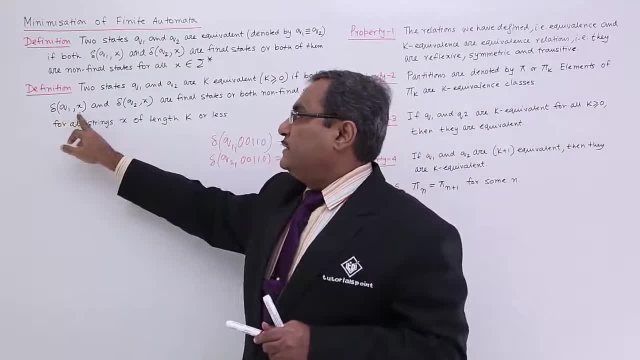 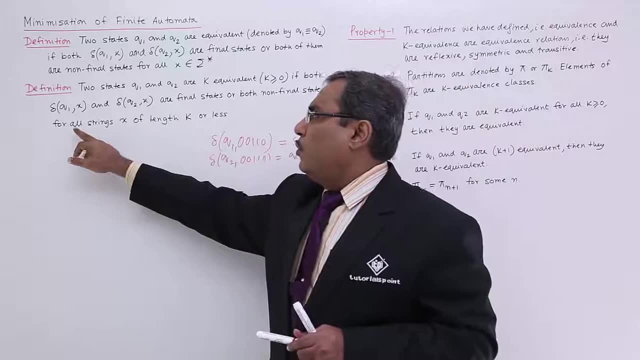 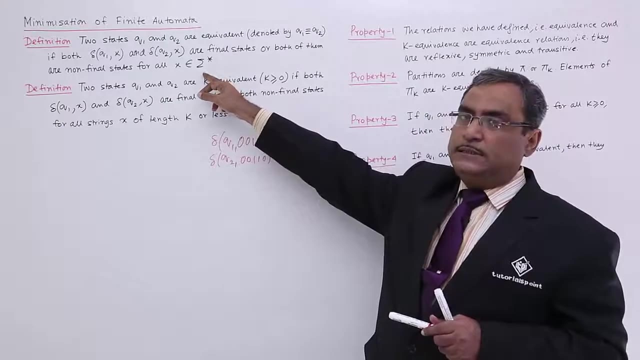 to 0.. If both delta q 1 x and delta q 2 x are final states or both non-final states for all strings of length k or less, Here we had, we had all possible strings. that means x belongs to sigma star, but here it is k equivalent. it will be known as a k equivalent. 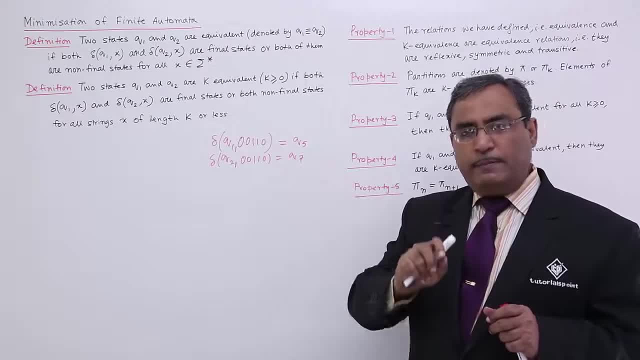 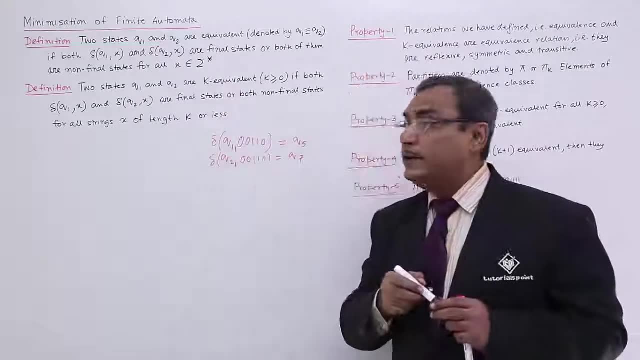 If the input string x is having a length either max to max k or less than that. So that is why it will be known as a k equivalent. It will be known as a k equivalent. So we are having this particular idea. Let me come to this particular part. 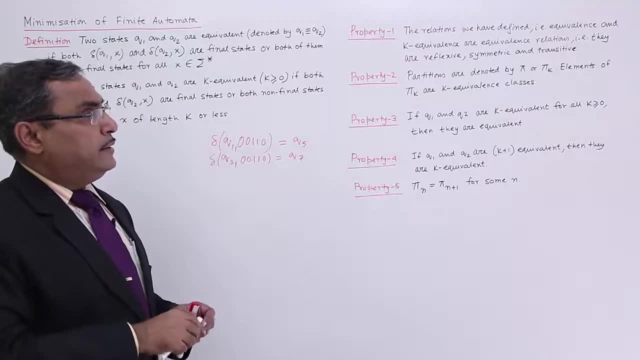 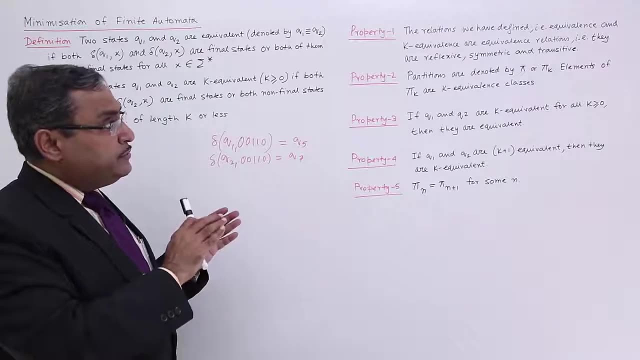 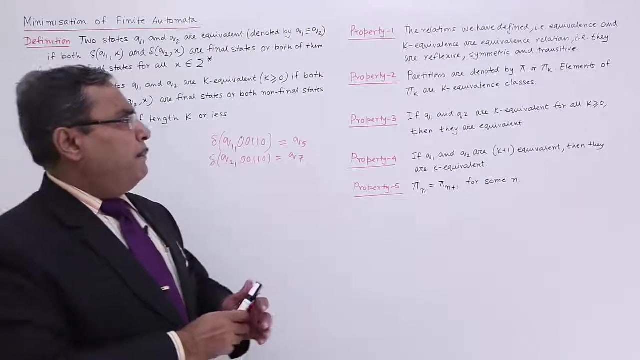 So now, the relations we have defined, that is, equivalence and k equivalence, are equivalence relations As they are equivalence relations, that is, they are reflexive, symmetrical and transitive Partitions are denoted by pi or pi k. Elements of pi k are k equivalent. 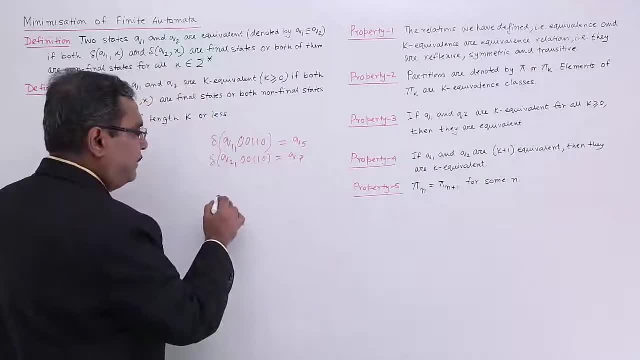 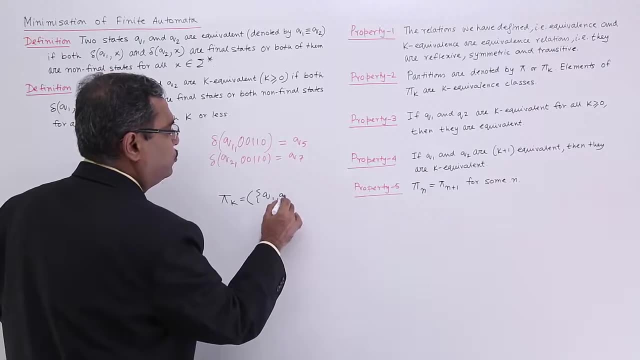 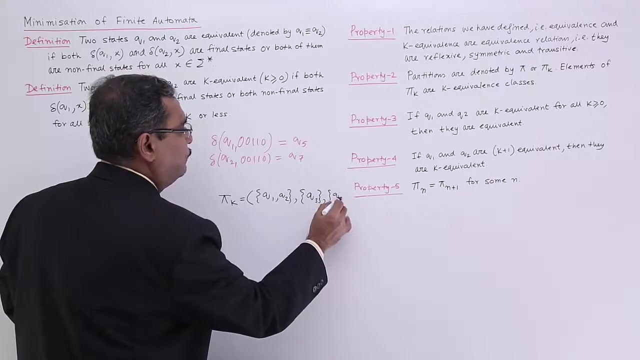 classes. In case of pi k. let us suppose we are having multiple number of states, Say, in case of pi k, we are having, say states say q 1, q 2, we are having state q 3 and we are having equivalent states say q 4 and q 5.. 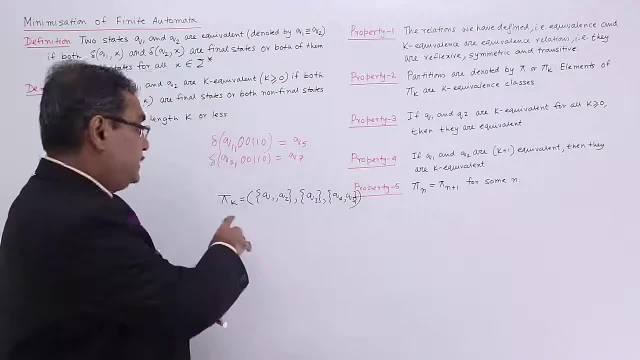 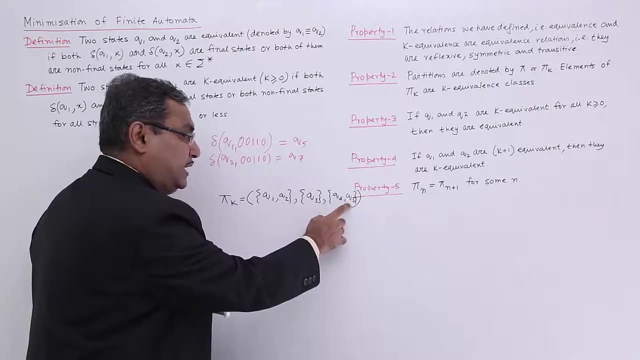 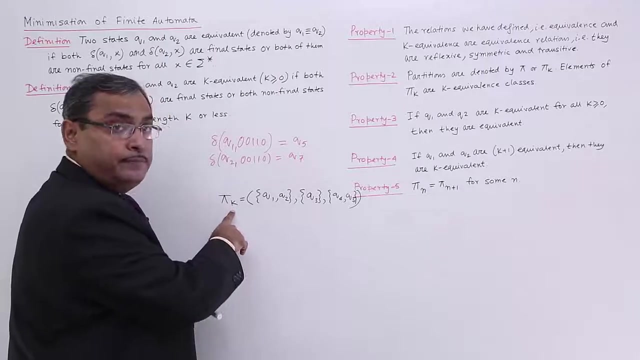 Now, if it is so, if it is so, that means it is pi k. that means these two states are k equivalent. These two states are k equivalent and it is a single state, So it is not having an equivalent to any other state. So that is a pi k. and what is a k equivalent We have? 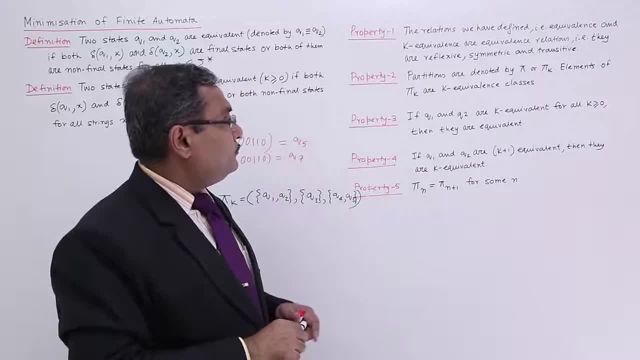 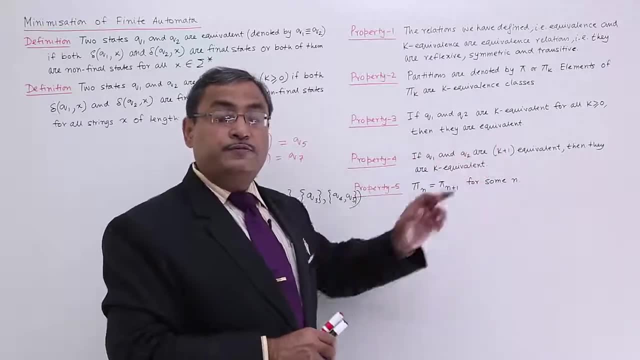 discussed that one here. Next one is that if q 1 and q 2 are k equivalent for all k greater than equal to 0, then they, then they are equivalent. That means for any value of k greater than equal to 0,. 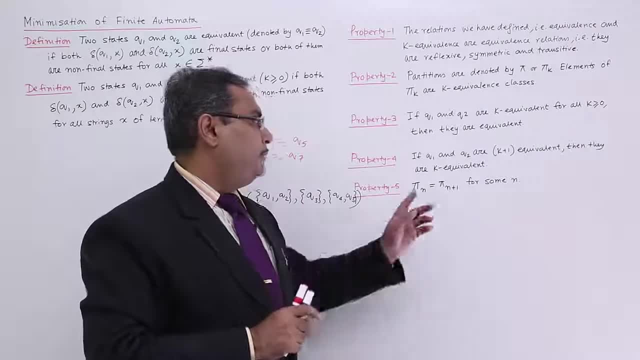 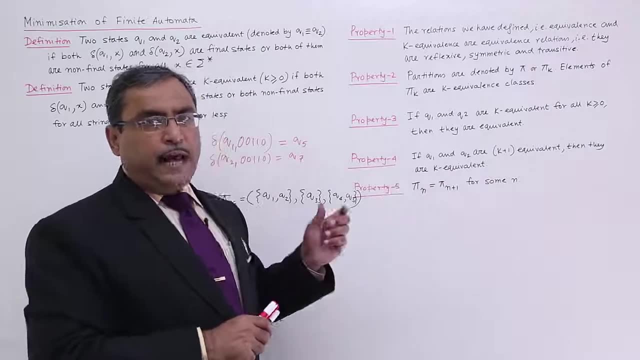 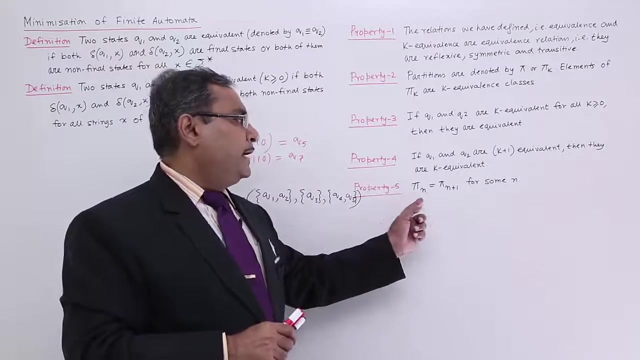 if they are equivalent, that means these two states are equivalent. If q1 and q2 are k plus 1 equivalent, then they are k equivalent. That means if they are having a, they are equivalent up to length 5, that means they are equivalent with length 4 also, And pi n is equal to pi n. 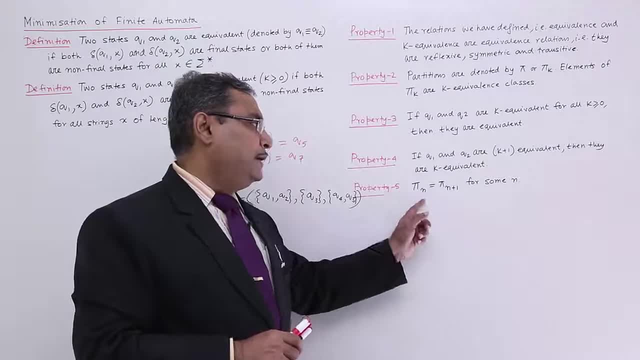 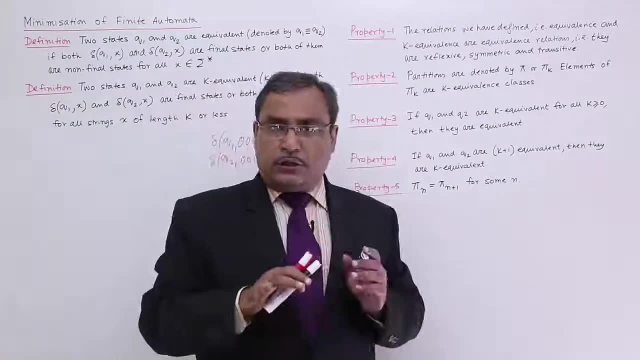 plus 1 for some time for some n I will be getting. pi n is equal to pi n plus 1 for some n. So whatever we have done the discussion here- if it is not clear to you, please watch the next. 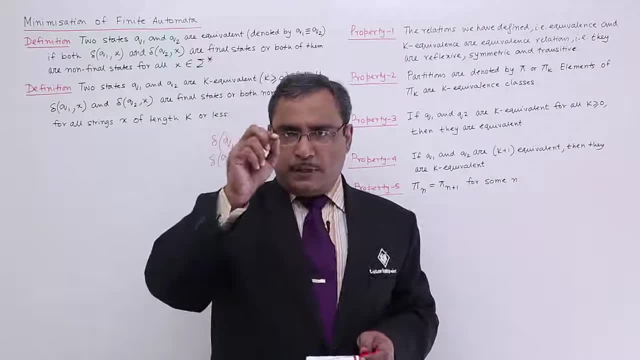 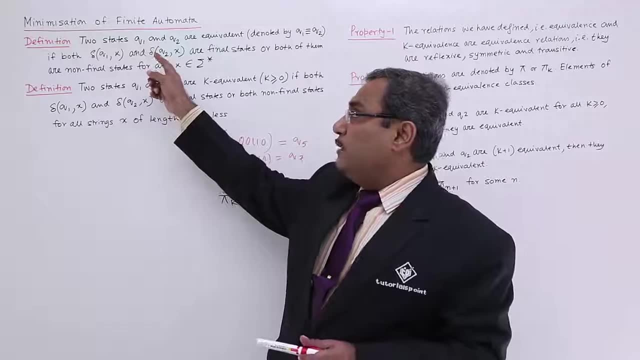 video where we have taken one example and we have- we have made that particular finite automata, minimized with each and every detailing, But there we will be using all these definitions, all these properties and all. Please remember them while watching that video. Please watch. 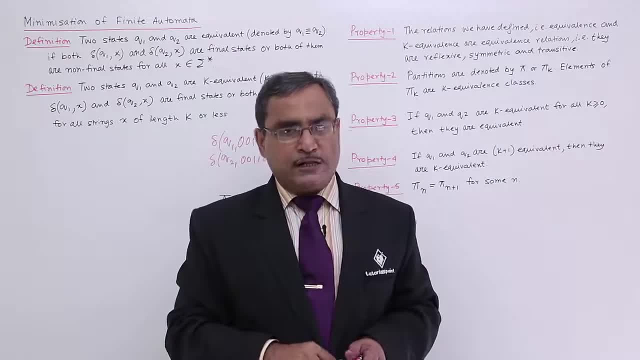 that one That will be in the continuation of this particular video. Thanks for watching this one.